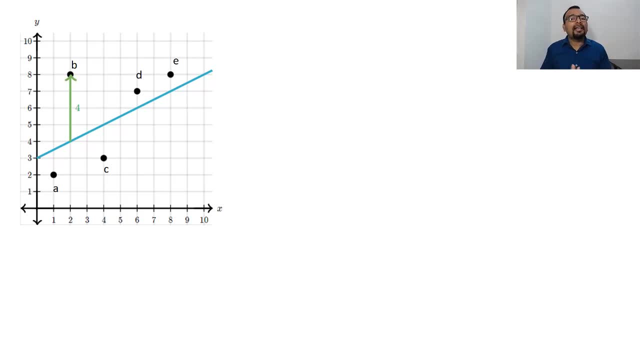 plotted against x-axis and the peak area is plotted against y-axis. and these are the five different concentration levels: Level A, B, C, D and E. So what you observe, that you know. for concentration B, the second concentration, there is a deviation in the response by four units. 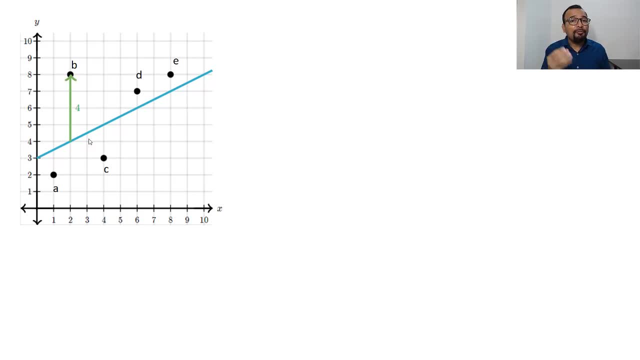 There is a deviation. There is a deviation for the response by four units against the predicted response. Now, whatever line you are seeing onto the graph is what is plotted in such a way that there will be a minimum deviation. There will be a minimum deviation between the observed responses. So what we 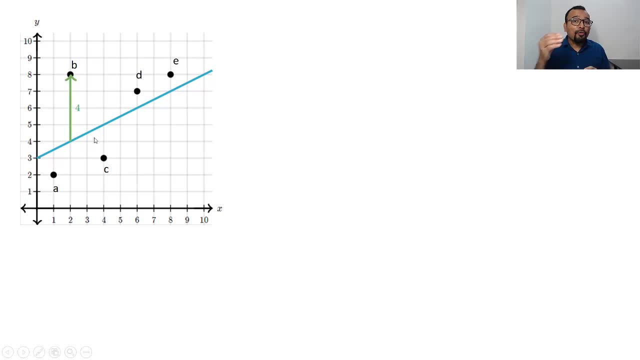 observe that for point B, the four unit is the observed deviation and this is nothing but the residual. This is nothing but the residual. So the residual for point number B is four and which is above the line by four units, which is the above the line by four units. So the vertical distance. 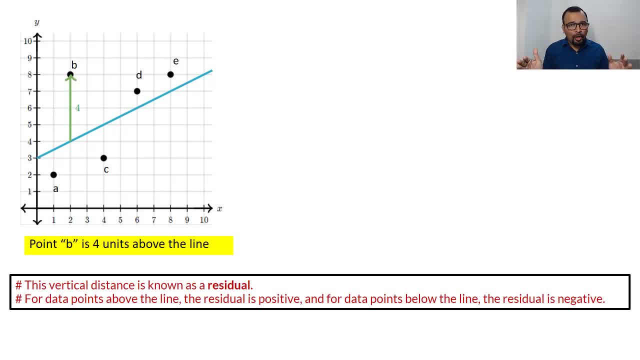 the vertical distance between your observed value and the predicted value is known as the residuals. The second important point is you know if the deviation is above the line, it is the plus deviation, The plus residuals, and if the deviation is below the line, it is the minus. 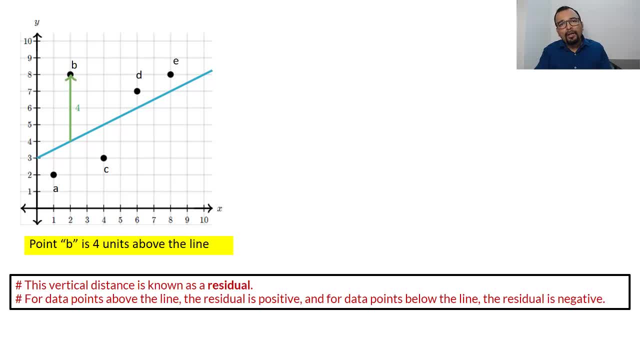 deviation. So let us understand the residuals with the help of another data point, and here in this case it is the concentration level C, and if you look at the deviation, you know is minus two. The deviation for the observed response at concentration C is minus two. 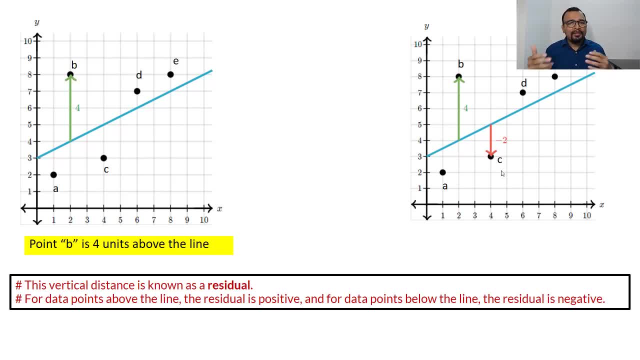 Below the line of regression. So this is called as the negative residual deviation. So we are going to understand what is the actual formula for the calculation of the residuals. right and sure it is so. so residuals is nothing but the difference between observed value and the predicted value. I 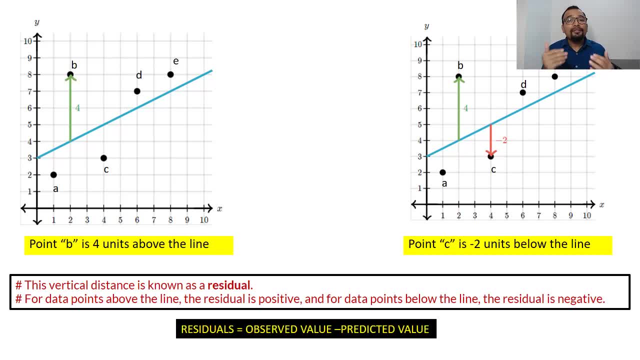 repeat once again, the residuals is nothing but the difference between observed value and the predicted value. So we are going to understand, you know, observed value is very much clear, to know that whatever response we are getting onto the peak area is nothing but our observed value, But how one can understand the 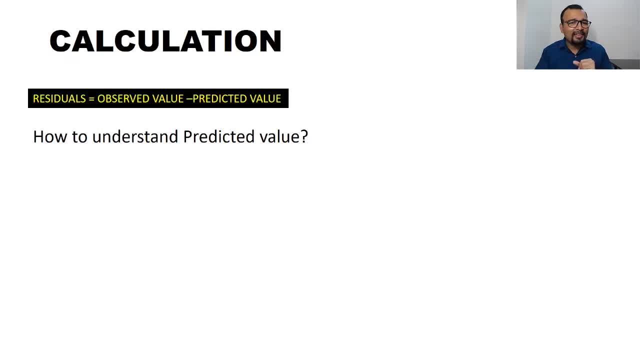 predicted value, And here is the solution for that. So, how to understand the predicted value? And we all know that the equation of linear line, the equation of linear line, is what y is equal to m, x plus c, And in this case, y is. 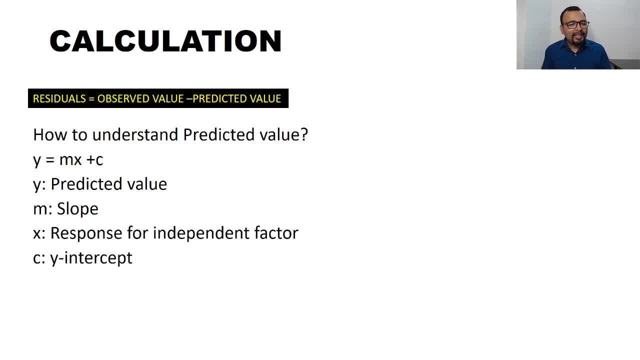 nothing but our predicted value. M is the slope, x is the response of our independent factor can be concentration, Then C is the y intercept. So let us understand, you know, the further simplified version of residuals is nothing but observed value minus. let us substitute this predicted value by m, x plus c and you will end. 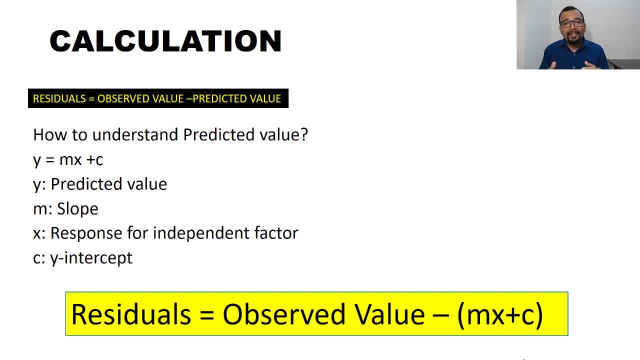 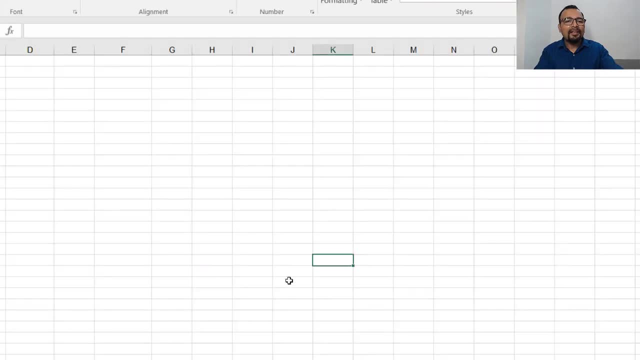 up getting the equation which is a residual is equal to observed value Minus in bracket m, x plus c. So with the help of this equation calculation formula, we are going to understand how practically one can calculate the residuals. And for that let me bring the excel sheet on the screen and let us 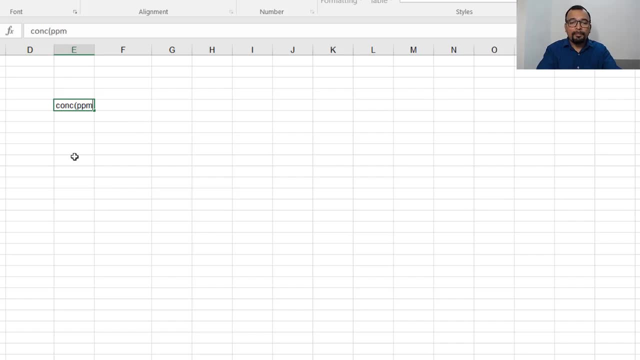 understand that concentration is in terms of ppm. and then there is a area right, there is a peak area for the linearity study. So let us assume that the concentration is 10.1 ppm, your first level. The second level is a 20.2 ppm. 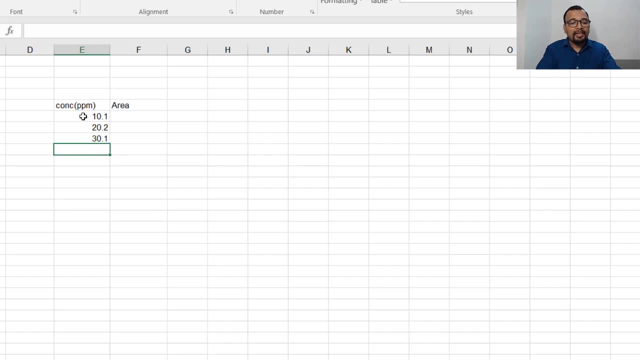 Third level is 30.1 ppm, Then the fourth level is 39.8 ppm and the last one is 50.5 ppm. I'm just taking the random values. Let us assume that the area observed for the 10.1 ppm concentration level is, let us say, 1000 ppm. 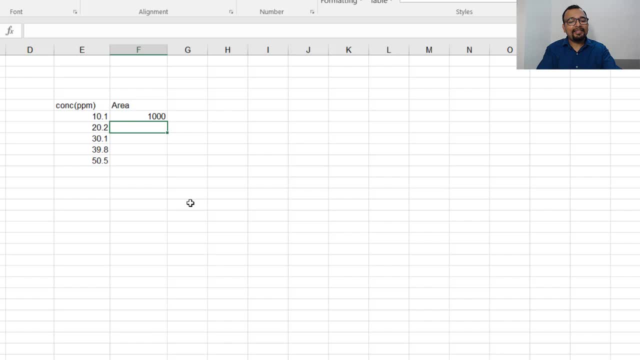 For the second concentration it is roughly 200.5.. For the third one it is 30.2 ppm, For third it is 40.55 ppm And for the last one it is 5.000 ppm. So these are the areas. So which one? what is the residuals now? 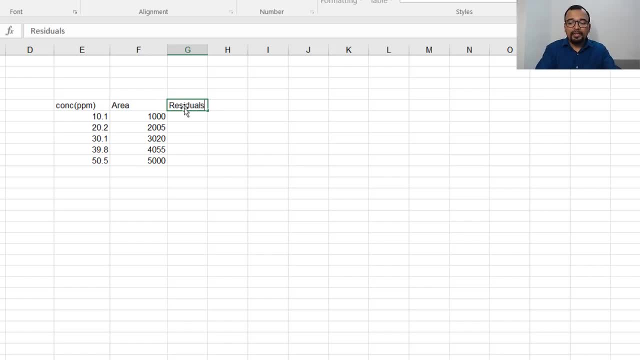 The residuals is. let me calculate the residuals. and the residuals for the second one is 10.7 ppm. is what the observed value minus the predicted value. so for calculation of the predicted value, we need to calculate the slope right, we need to calculate the slope and y intercept. okay, 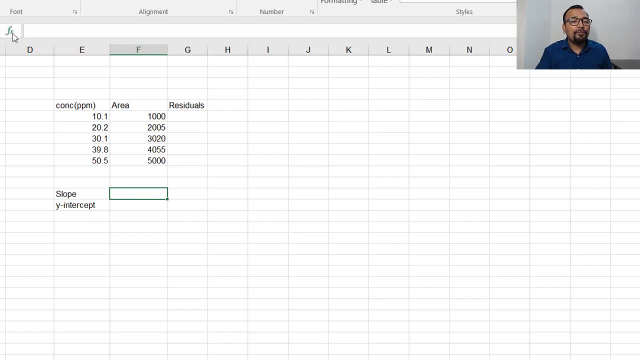 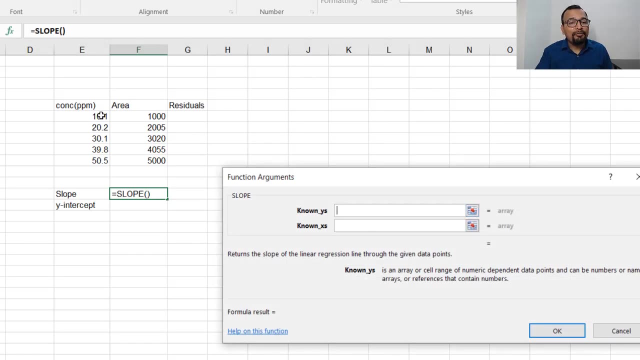 so let us calculate slope quickly with the help of excel functions. and here is the function for slope right: the y is what is the independent values and what is the independent values? concentration is the independent values and x is what? uh, sorry, i, i made the mistake. so in case of y, it is the uh. 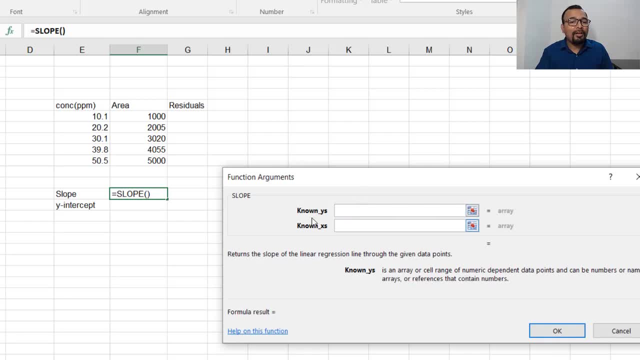 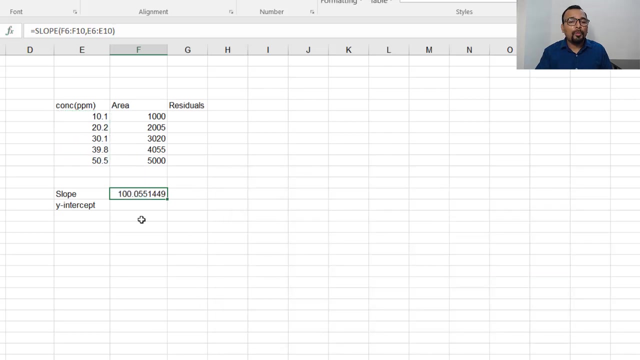 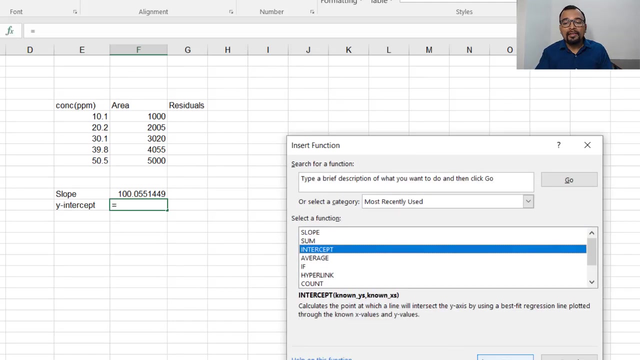 it is the dependent values. y is the dependent values and we know that the area is dependent on to someone, that is the concentration. so area becomes dependent value and x becomes the independent value, which is the concentration. so this is the slope: hundred point zero, double five, and let us calculate the y intercept. okay, the intercept. so again, y is the independent values. so 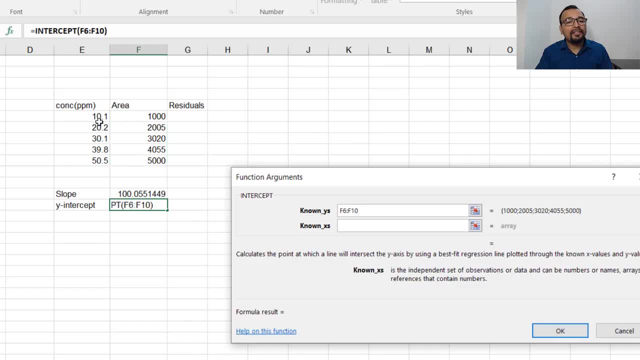 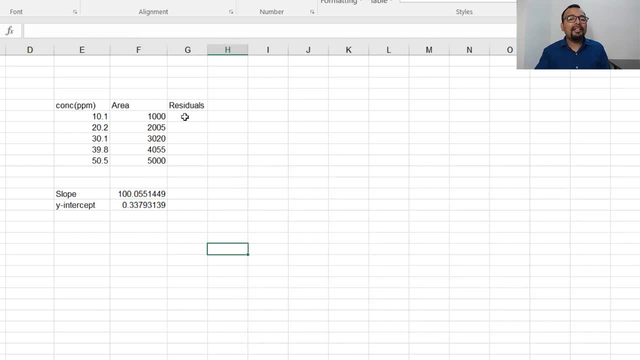 area is always dependent on to the concentration. so x becomes the concentration and here is the y intercept. so we got the required values now. so residence is for the observed value. okay, what is the observed value? is the area hundred one thousand, in this case, minus mx, plus c? what is the m? m stands for the slope, m stands for the slope and. 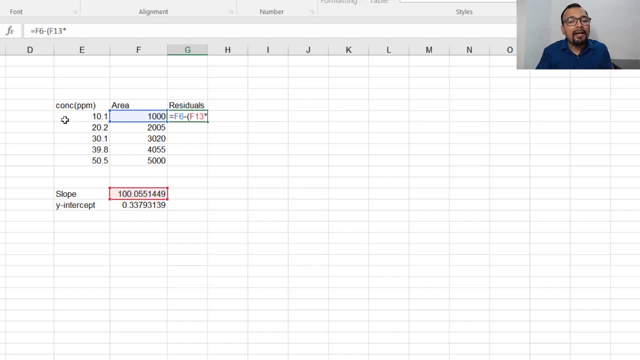 into x stands for the uh dependent value, that is the concentration, in this case plus plus. the intercept is nothing but here and here is the david: the residuals, right residuals for first point, that is minus 10.8949. so this is the deviation in the area. 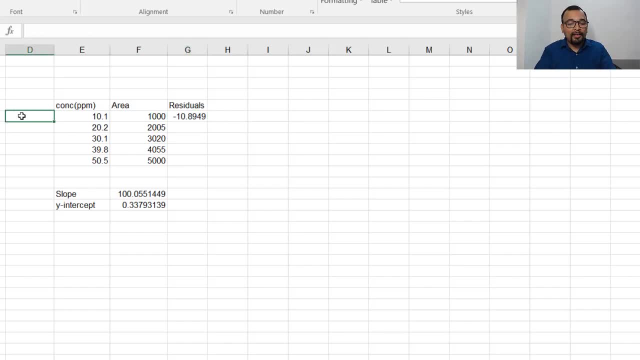 observed for the first level, that is, l1. so we will say this: l1, linearity, level 2, l3, then l3, l4 and then l5. so let us do a small rearrangement. that: what are the constant values over here? right, this f6 is going to change, but the slope value is going to remain constant throughout. 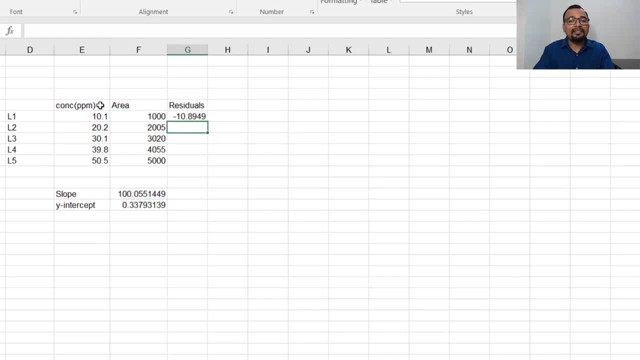 all. so let us put this dollar symbol across this, and similarly, the y intercept is also going to remain the same, and i have put the dollar symbol across it, so just drag it and you will get the residuals for all these five levels right. the next is what? the residual sum of the squares? 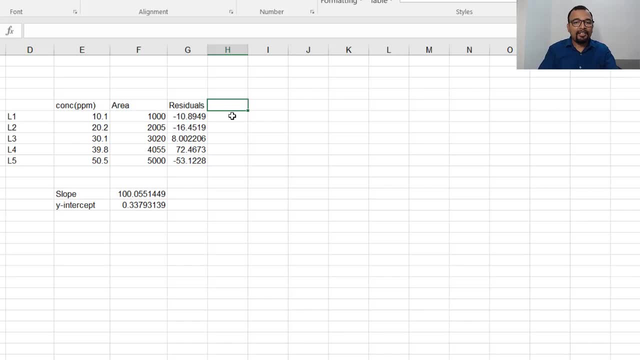 so you need to first first calculate the square, residual square, residual square. and how to calculate that? okay, you have to just put sine is equal to this into again this right same, the same row, and you will get the square of that. so this is the square of the residuals and then finally, the sum of. 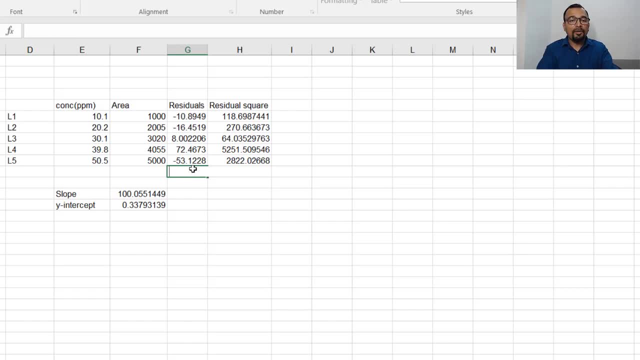 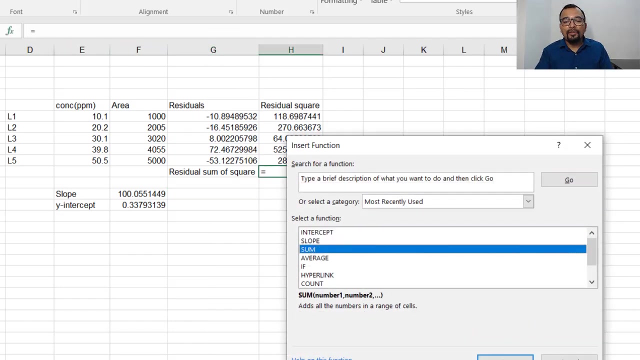 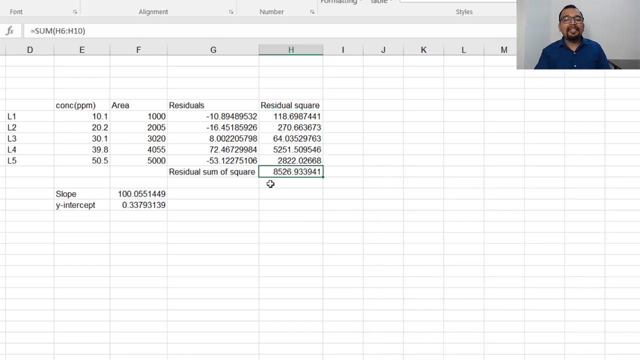 residual sum of squares. so, residual sum of squares. okay, and here is the summation. let's just do the summation of all the residual squares and you will get the value for a residual sum of squares. so this is the value that you was looking for. right for calculation of estimation of the sum of squares. 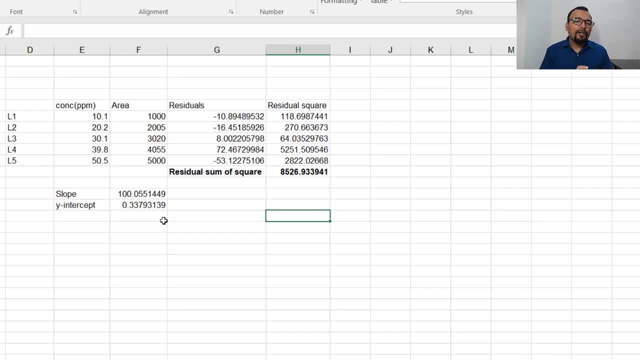 of one of your linearity parameter. so if you look at the uh residuals, you know the summation of all the residual values will always be 0. if you add this, you will end up getting the zero value right. this is the uh, the property of the residuals, and that is what you know. the regression line is: drawn in such a way to see that this is the, the? u star should be equal to the t t else. so you need two things: on the left, one negative eleventh, and on the right, one negative out, and so we are. Was the sinarpine is the sum of theound, the element of the squadron, and so we keep selecting. this has a frequency, and then after that, 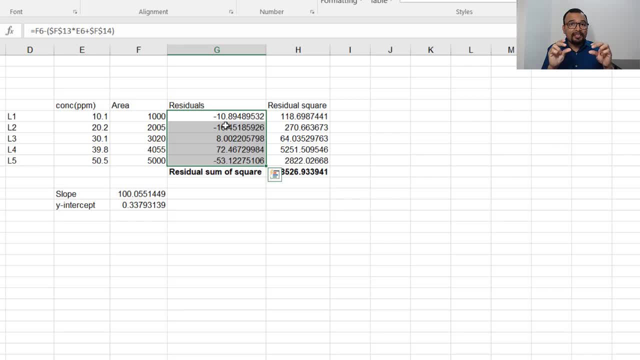 that the distance, the distance, the difference between the distance from each point, will be as low as possible. so this summation of residuals is always should be close to zero. so you got the residuals, then the square of the residuals and then the residual sum of the squares. so i hope.